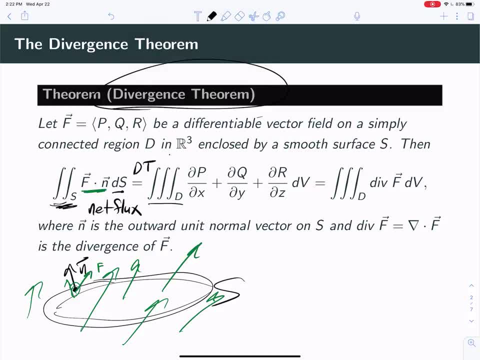 and the divergence theorem says: hey, you can instead integrate the divergence of the vector field, the divergence of the vector field inside the surface. So if you take each point in the solid- not on the surface, but in the solid- and compute its divergence, 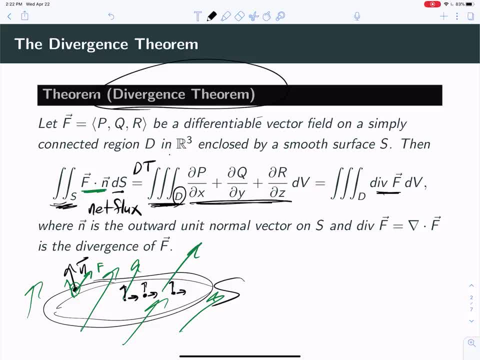 compute its divergence, compute its divergence, then what happens is the sum of all these individual divergences inside the solid is equal to the net flux out of the surface, because, of course, these divergences cancel. these divergences cancel, and the only ones that don't cancel are the ones that are sort of on the edge of the solid, on the boundary. 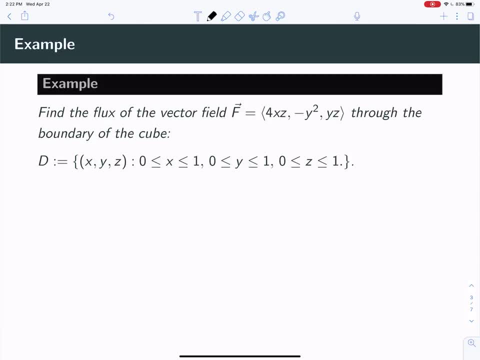 Okay. so a typical problem then is going to say, hey, find the flux of N, this vector field, through the boundary of the cube. and then you'd say, okay, well, I've got to do a surface integral. They're asking for flux, so I would do f dotted with n? ds, and that's going. 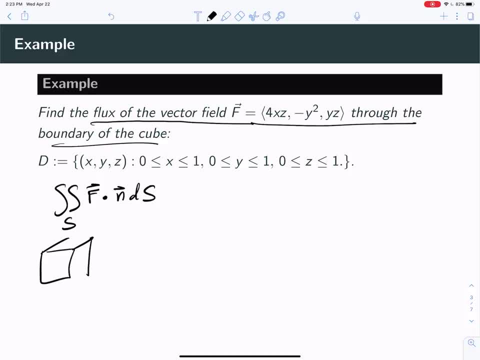 to be some complicated surface integral, because this is a cube, It's actually going to have six boundary surfaces. so this is actually six boundary surface integrals. but no, no, no, You can use the divergence theorem to say, instead, I'm going to do a triple integral on the solid. 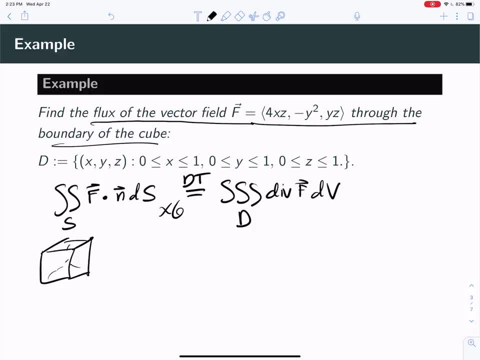 where I just integrate the divergence of the vector field dv. and in this case, because the solid is a cube, I'm just going to integrate the z's from 0 to 1, and the y's from 0 to 1,. 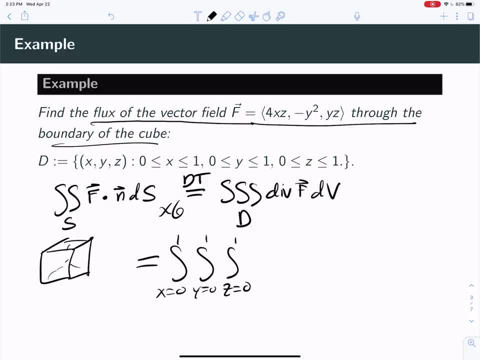 and the x's from 0 to 1, and inside the integral we put the divergence of the vector field. so we take the x derivative of 4xz, that's 4z. We take the y derivative of the y component, that's negative. 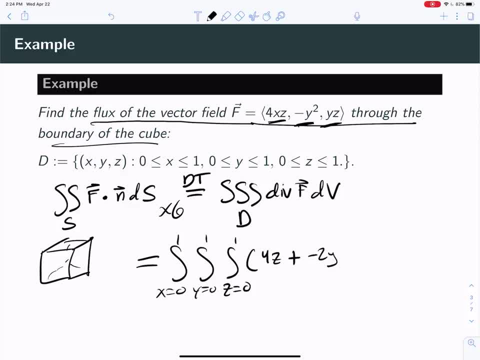 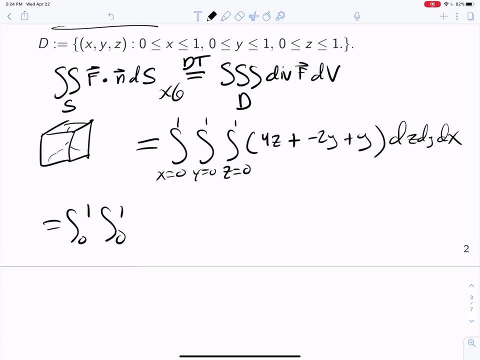 2y and we take the z derivative of the z component, that's y, dz, dy, dx, and now we've just got a nice triple integral waiting for us to compute. So let us compute it. then We're going to have 4z When we 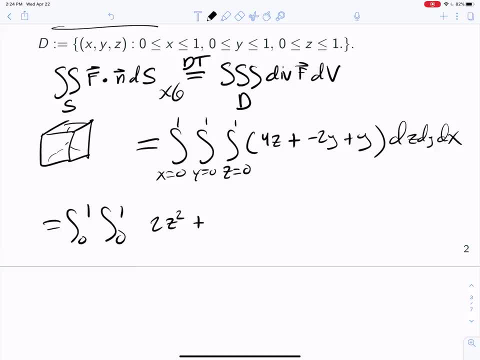 integrate 4z, we're going to get 2z squared and then we're going to have: let's see, this is minus y, so minus yz when we integrate it with respect to the z derivative of the z component. So we're. 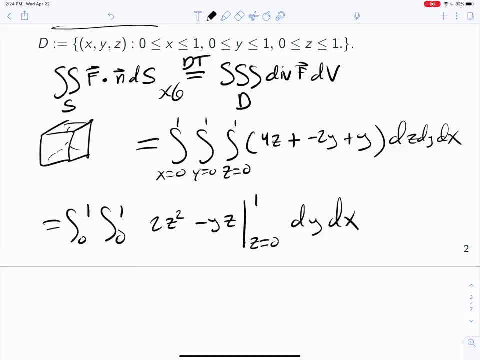 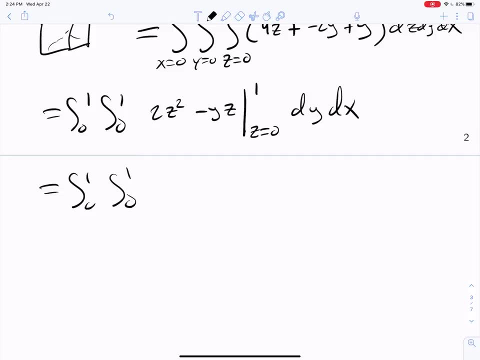 going to get 2y minus y, squared over 2, evaluated from 0 to 1, dy dx. and when we do that, we're going to get what? Plug in 1, we'll get 2 minus y, and plug in 0, we're going to get 0 minus 0, dy dx. 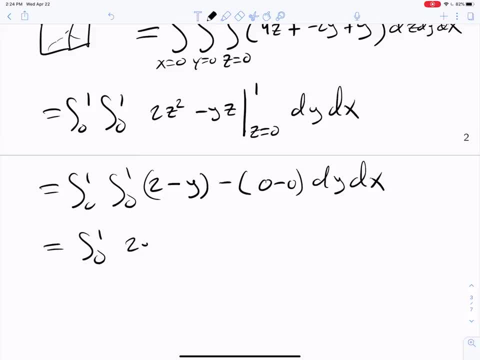 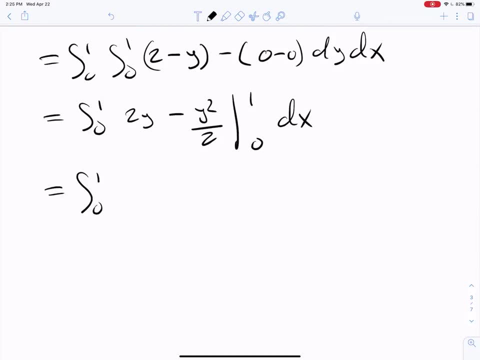 Okay, and now we'll integrate the y's. We're going to get 2y minus y squared over 2, evaluated from 0 to 1, dx, And if we plug in 1, we're going to get 2 minus a half minus 0 minus 0, dx, and that gives us 3. 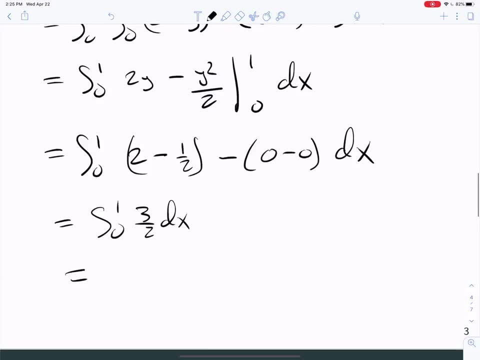 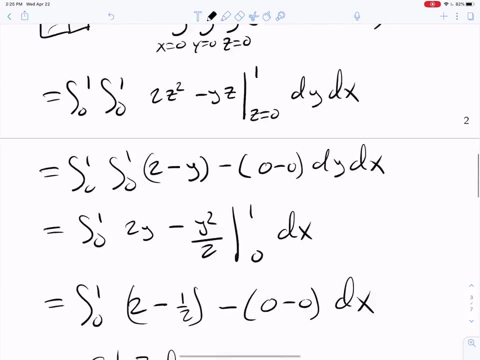 halves dx, and now we integrate the x's and we get 3 halves x, evaluated from 0 to 1, which is 3 halves. That's the final answer. So the flux through the surface is 3 halves, but we didn't. 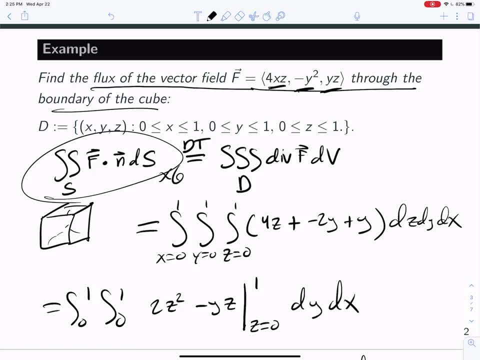 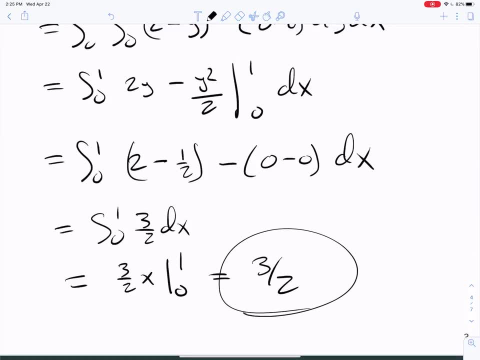 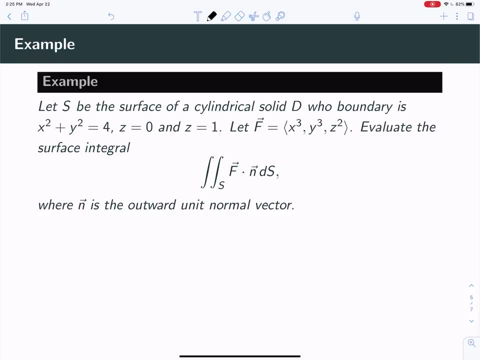 have to do 6 surface integrals. we just did a single flux through the surface and that's the whole triple integral on the solid, where we integrated the divergence of that vector field. Alright, let's tackle another one. Let s be the surface of the cylindrical solid d, whose boundary 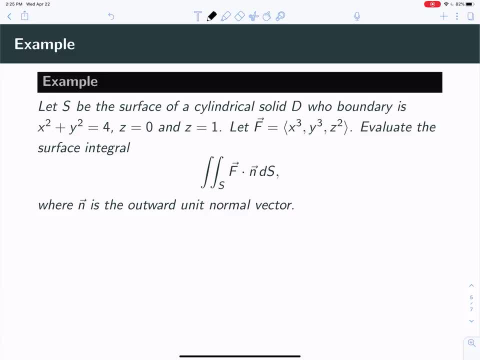 is x squared plus y squared equals 4,, z equals 0, and z equals 1.. Okay, so we've got a cylinder here. looks like that there's z equals 0,, there's z equals 1, and this is: 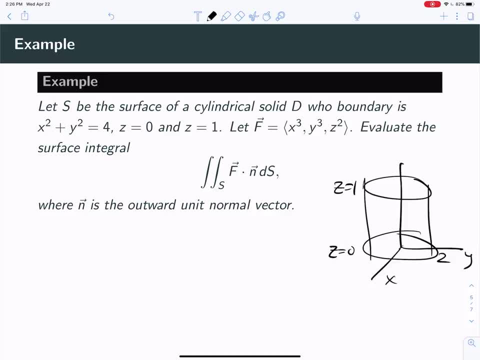 the cylinder, x squared plus y squared, equals 4, so that's a circle of radius 2.. And if you were going to compute this flux integral through the surface, you'd actually have to do 1,, 2,, 3 surface integrals. 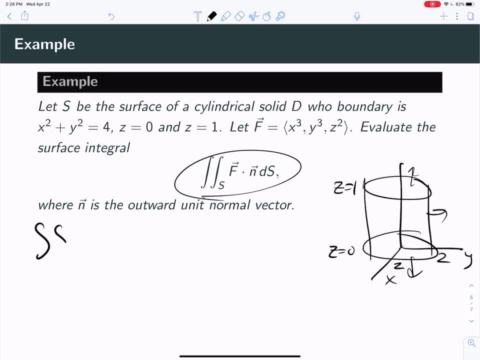 because there's 3 different surfaces. but are we going to do 3 surface integrals to find the flux through that surface? No, we're going to use the divergence theorem. and the divergence theorem is going to just say: hey, do you want to find the flux through that surface? No, we're going to use the. 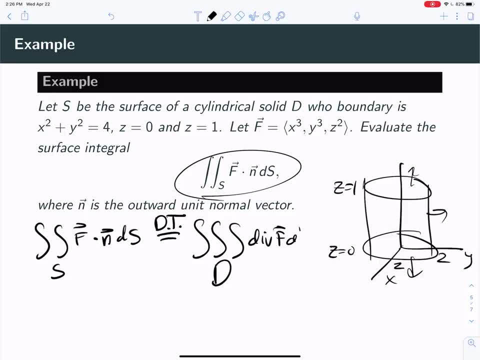 2 surface integrals and do a triple integral on the solid d of the divergence of the vector field dv, and that's all we have to do. Okay, so to do that, then we're going to need to know what is the 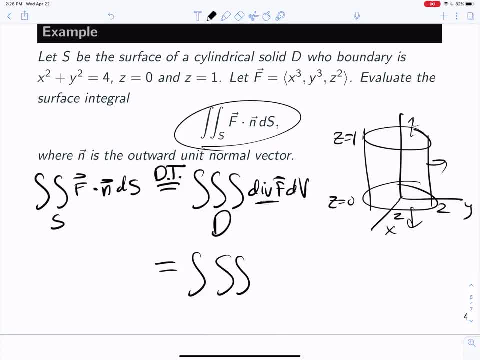 divergence of the vector field. so let's take a look. what is that divergence? Well, here's the vector field f. So we take the x derivative of x cubed, that's 3x squared. We take the y derivative of y cubed, that's 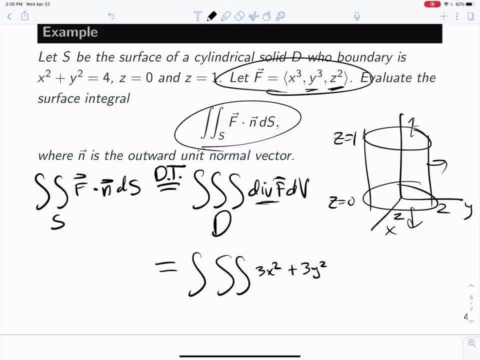 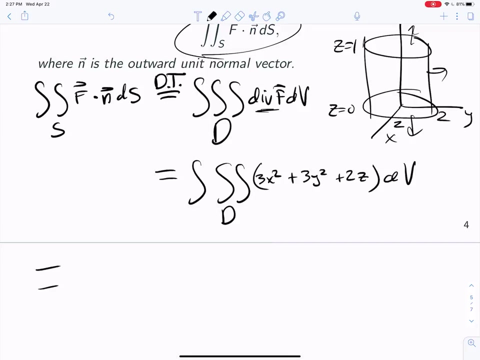 3 y squared, And we take the z derivative of z squared, that's 2z, and we integrate that on the solid region D. Okay, now this is a cylinder, so I'm thinking probably cylindrical coordinates might be nice. So if we did that, we're going to turn this into Zs from 0 to 1, it looks like. 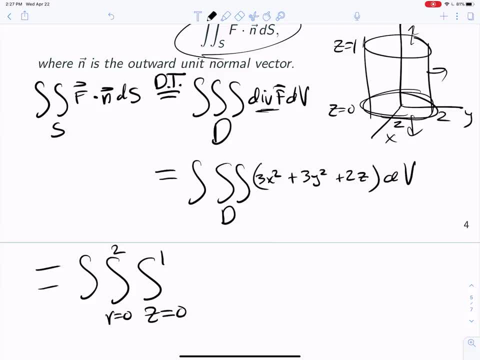 Rs from 0 to 2, because that's a circle of radius 2, and then thetas from 0 to 2 pi. the function we're integrating is 3r squared, because that's x squared plus y squared, is r squared plus 2z. 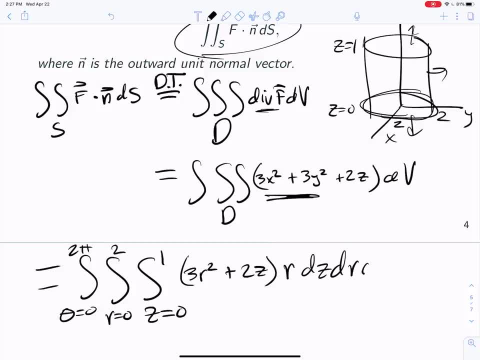 and then we have r, dz, dr, d, theta, that's dv in cylindrical coordinates. Okay, so now we've just got a triple integral. we have to work it out, but we're going to get the answer, no problem. 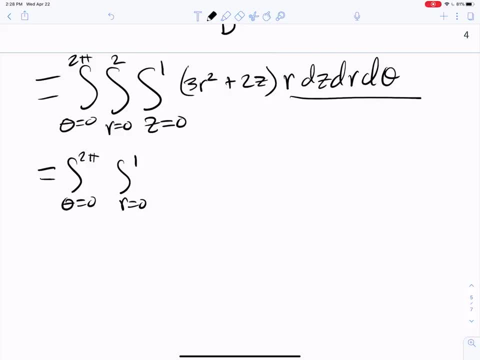 So let's integrate the Zs first. that's going to give us 3r cubed z plus rz, squared evaluated from 0 to 1, I just took that r, multiplied it in to r squared and to 2, and then integrated z to get z squared and integrated 3 to get 3z. 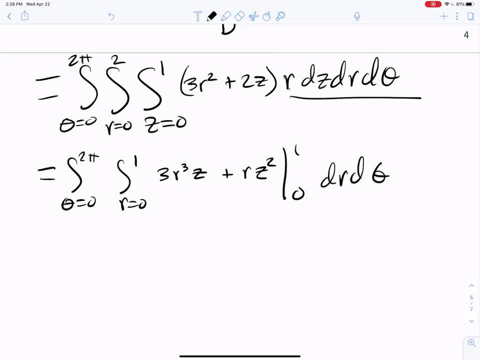 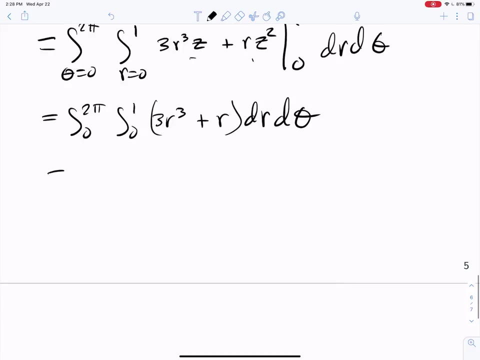 and then I'm going to evaluate that from 0 to 1, and when I do that, I'm going to get 3r cubed plus r, and then 0 minus 0 is 0.. Okay, dr d theta, now let's integrate the r's. 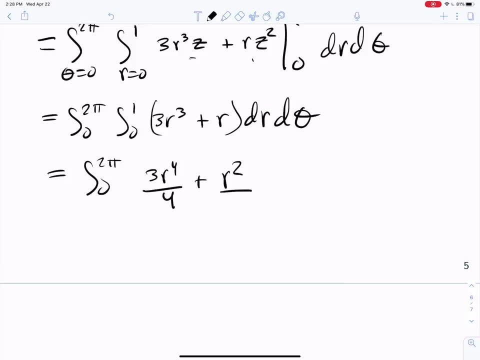 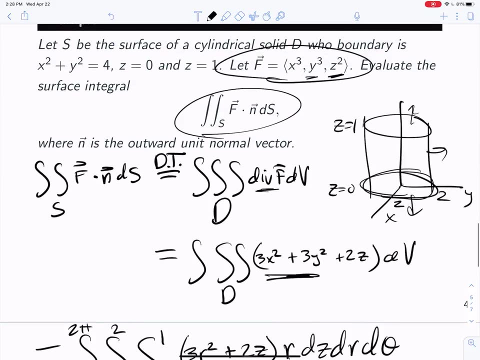 3r to the 4 over 4 plus r, squared over 2, evaluated from 0,, not 0 to 1, I think this was the circle of radius 2, wasn't it? Yes, Okay, the circle of radius 2,.